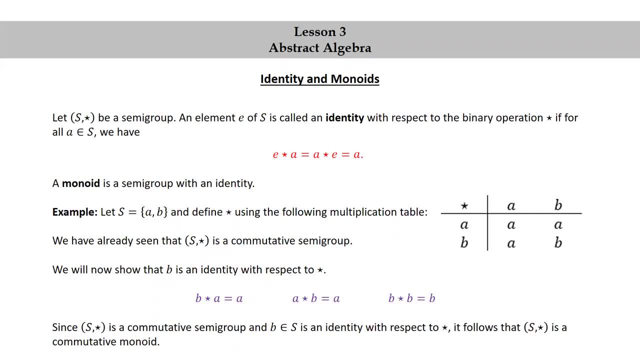 Since S-star is a commutative semigroup and B and S is an identity with respect to star, it follows that S-star is a commutative monoid. Notice that the row corresponding to B is the same as the input row. 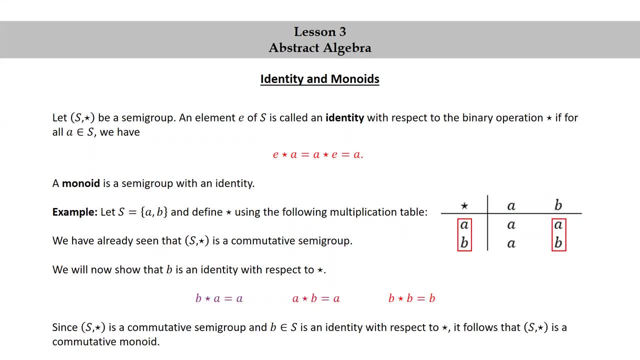 Also, the column corresponding to B is the same as the input row. Notice that the row corresponding to B is the same as the input column. 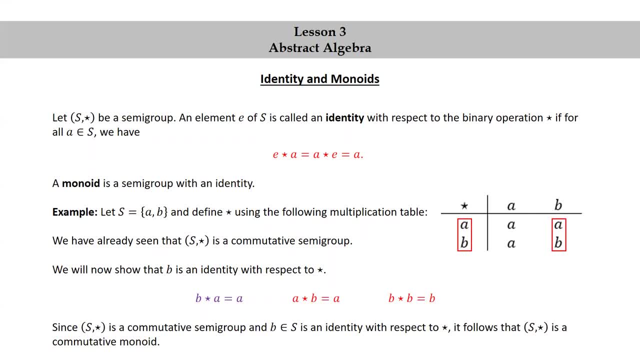 This is a nice visual way to use the table to recognize that an element is an identity. 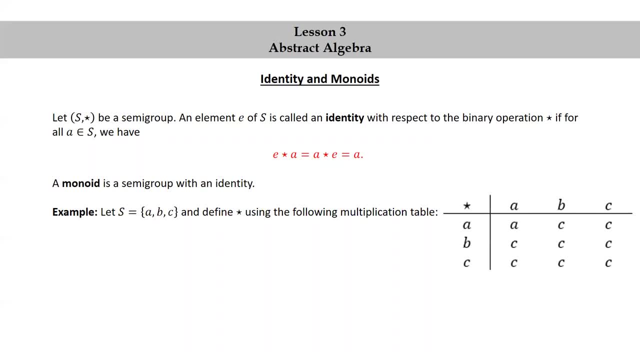 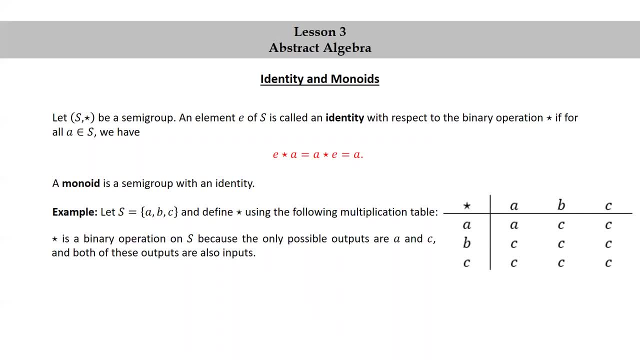 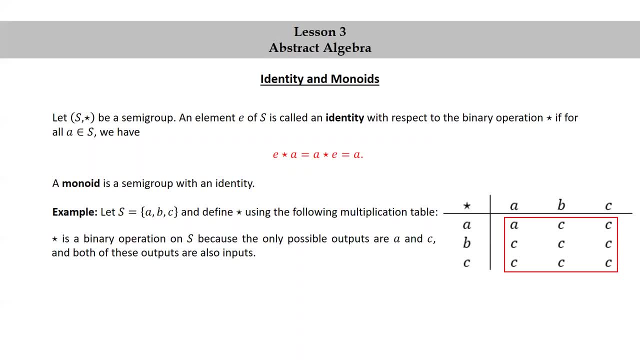 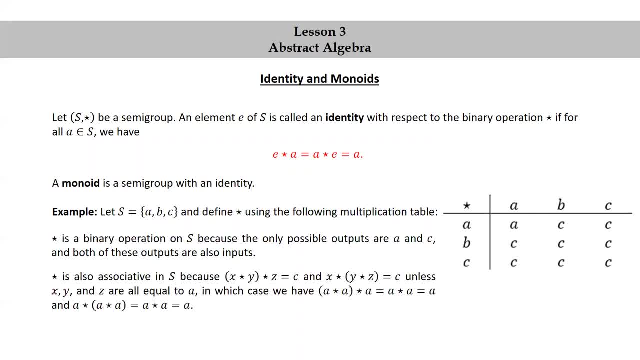 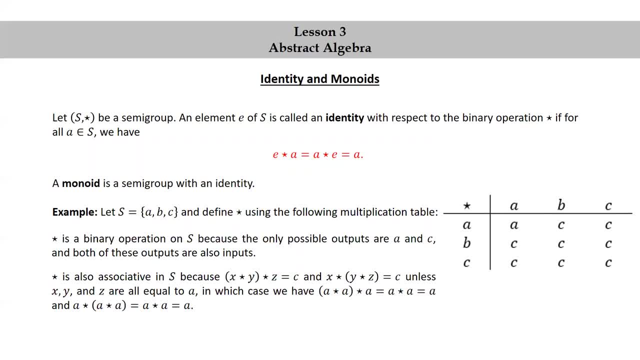 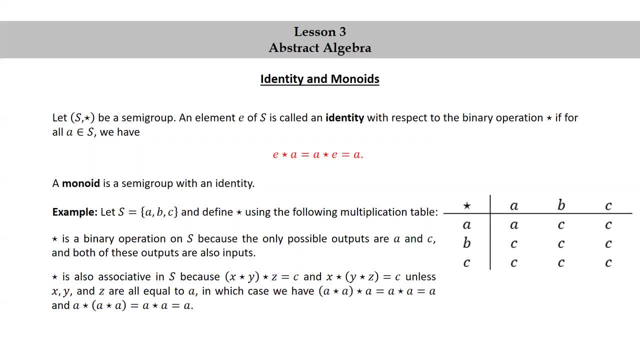 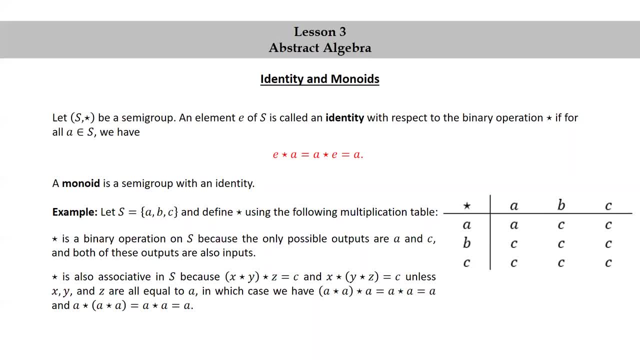 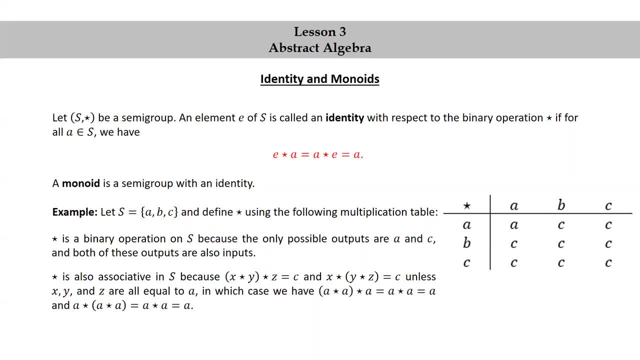 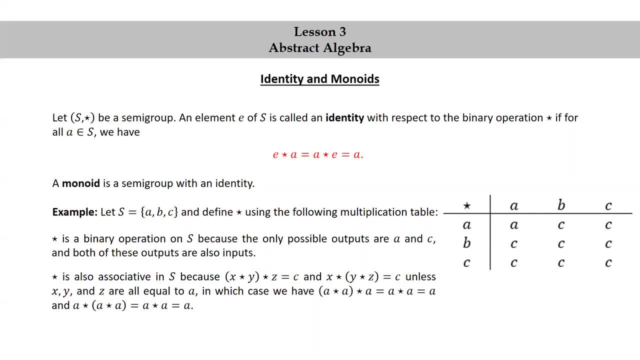 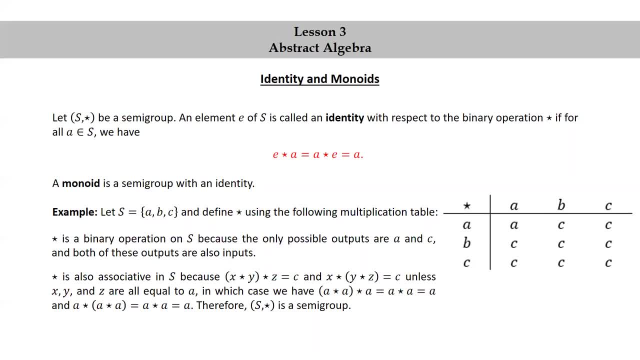 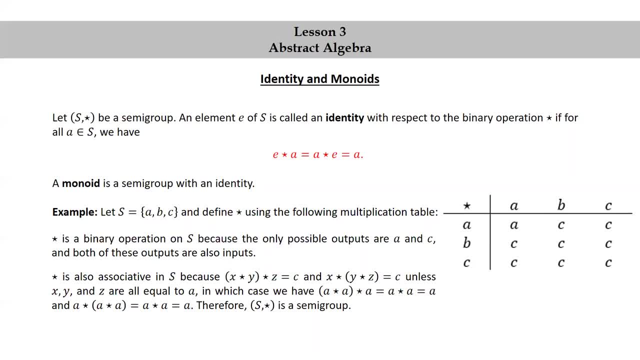 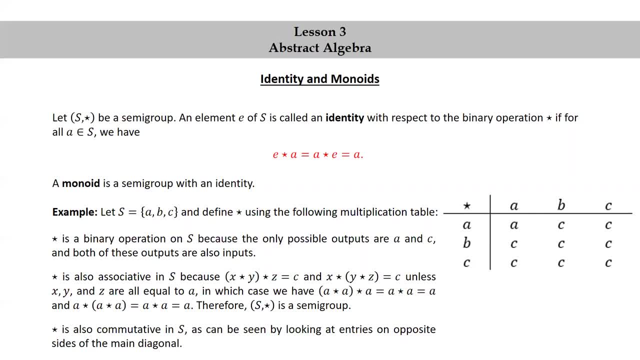 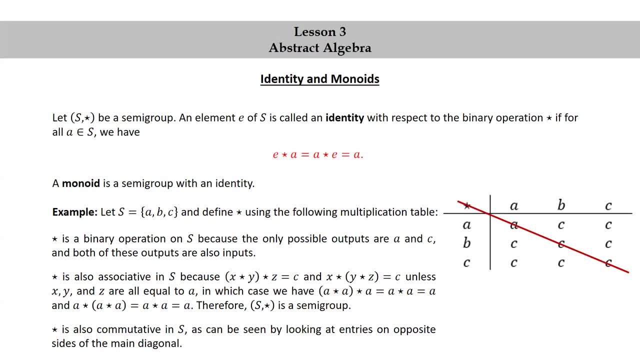 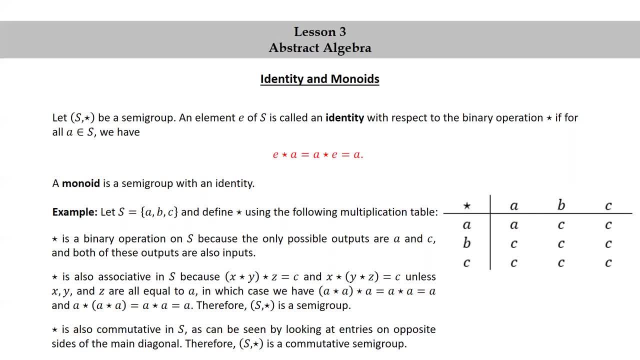 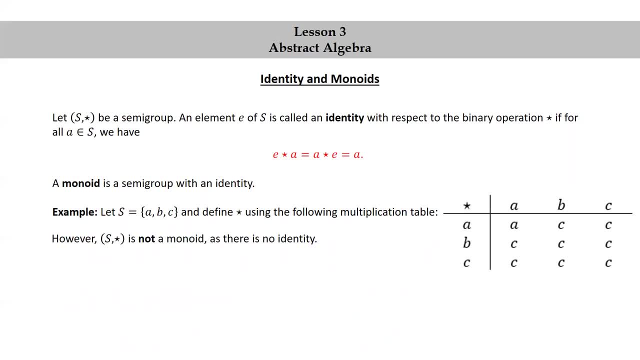 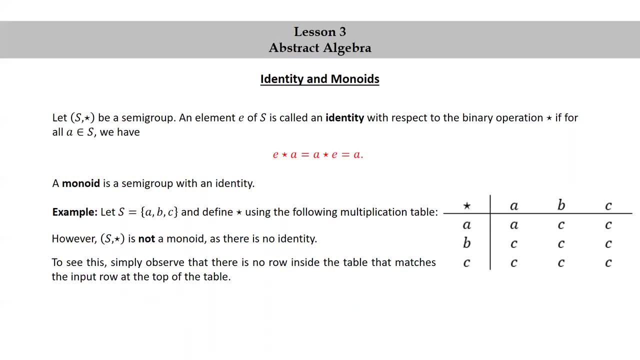 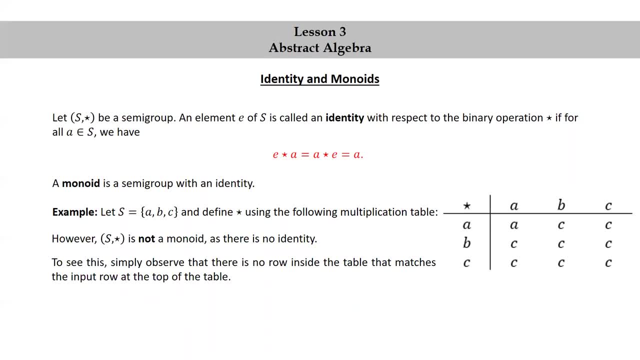 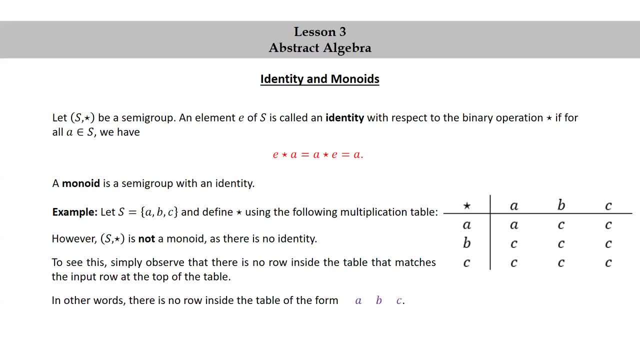 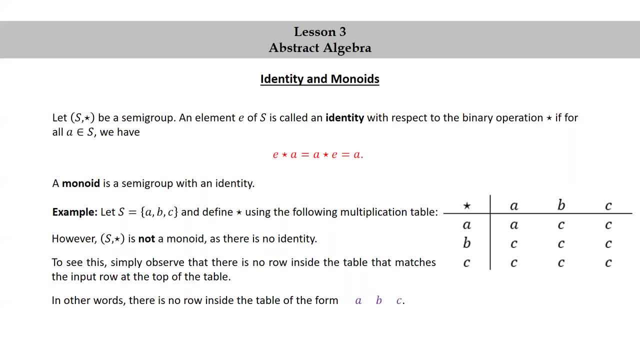 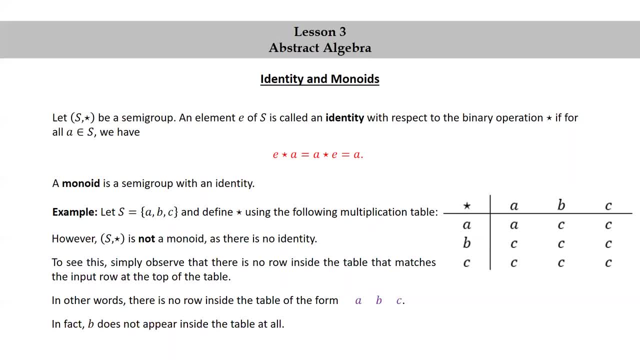 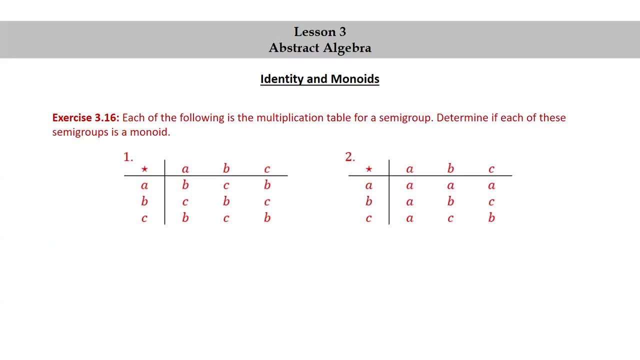 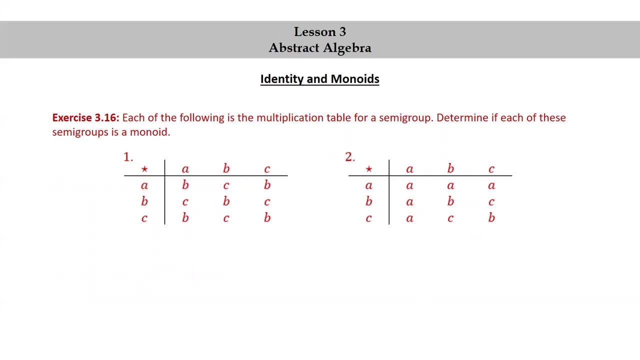 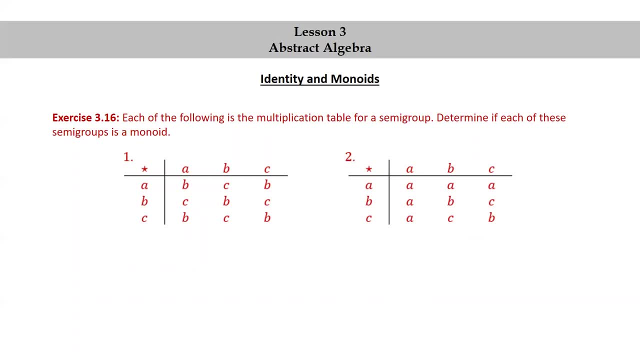 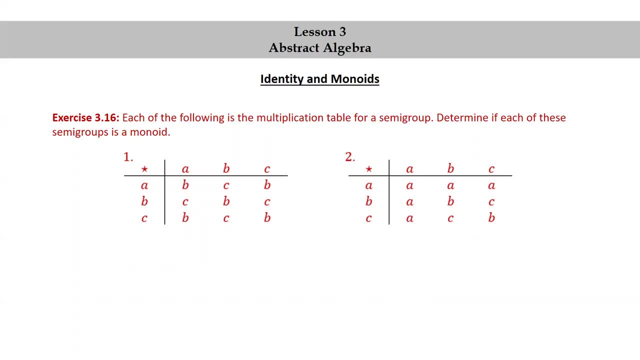 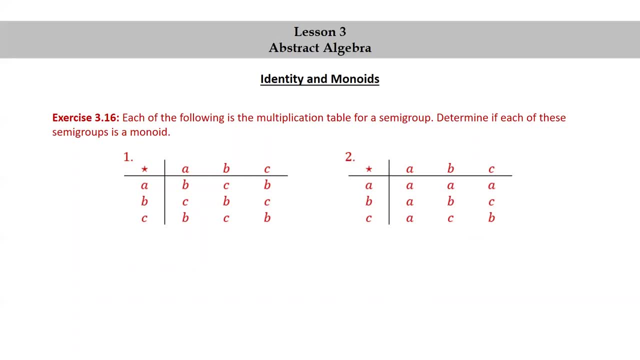 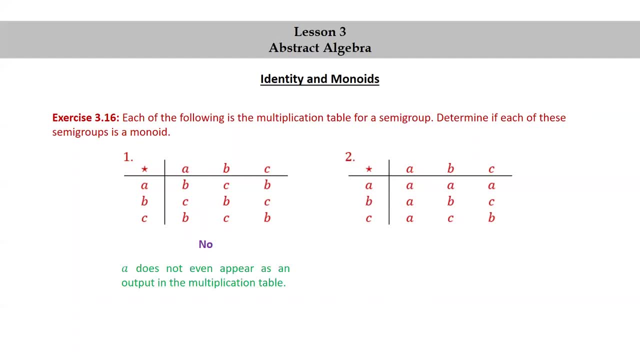 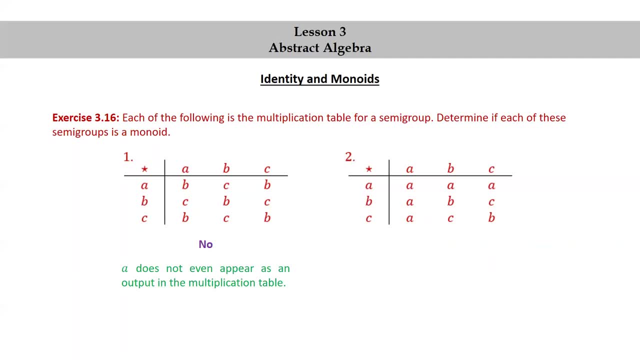 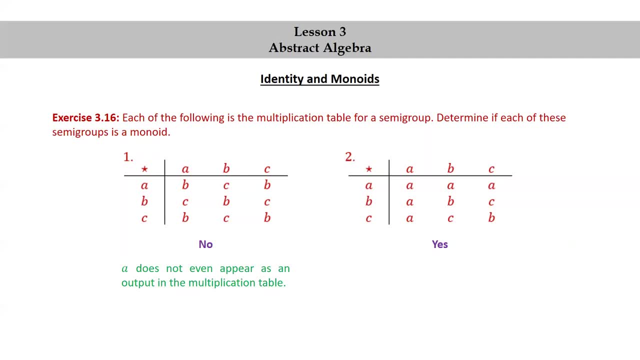 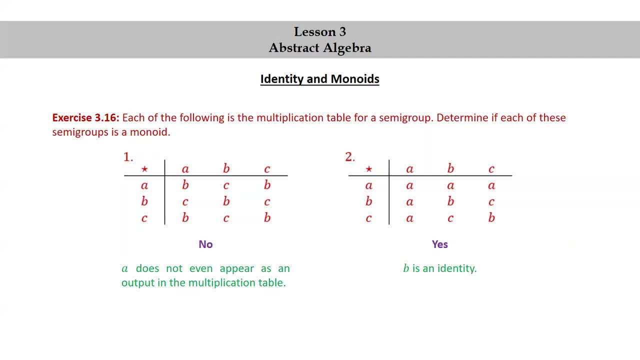 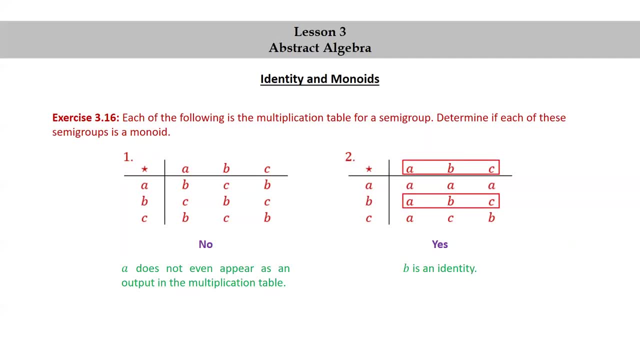 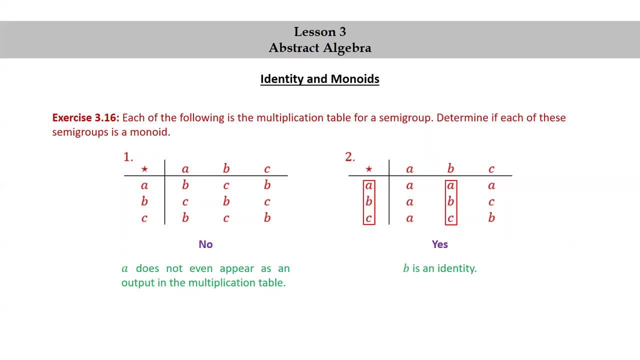 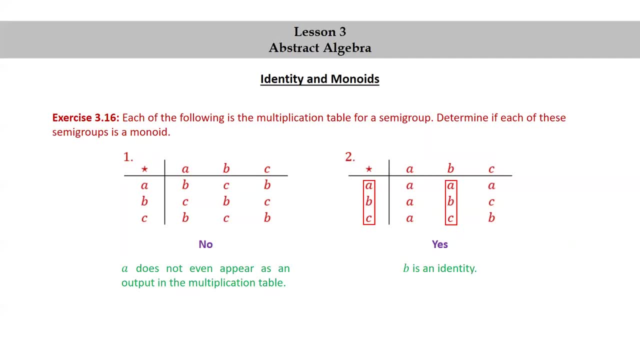 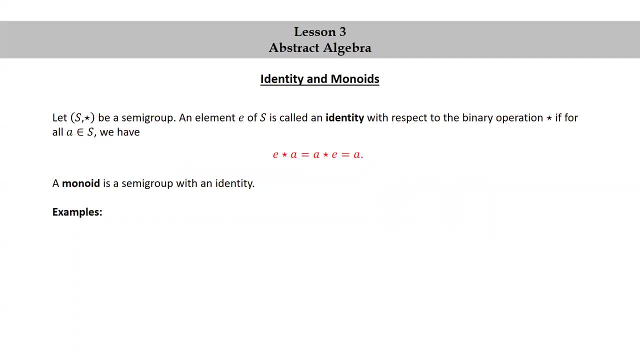 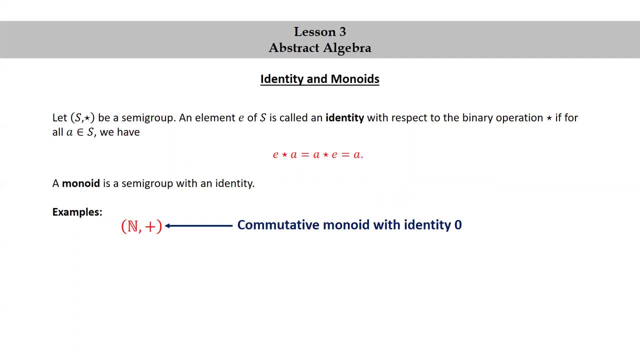 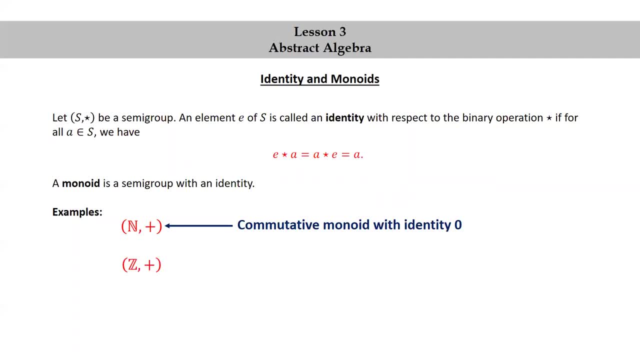 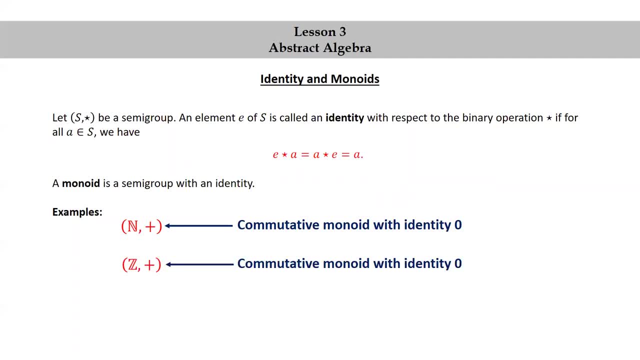 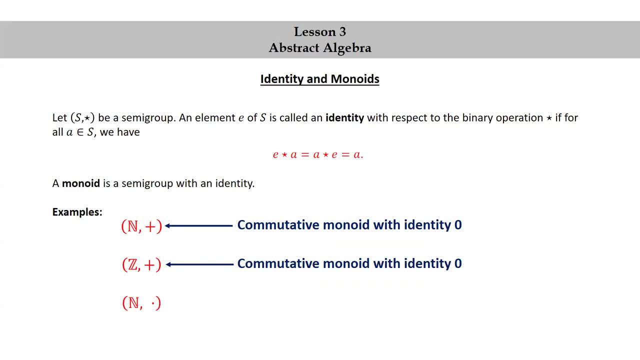 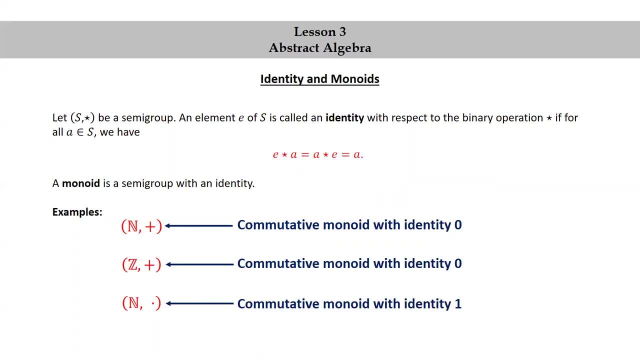 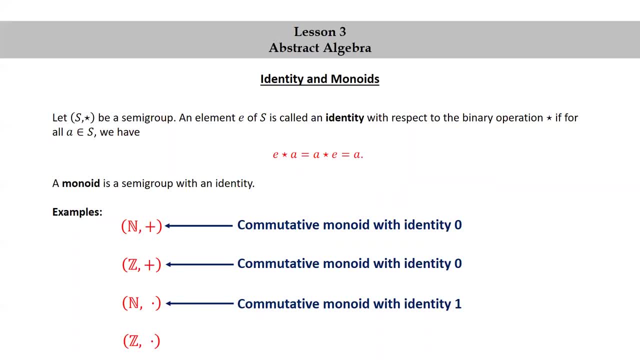 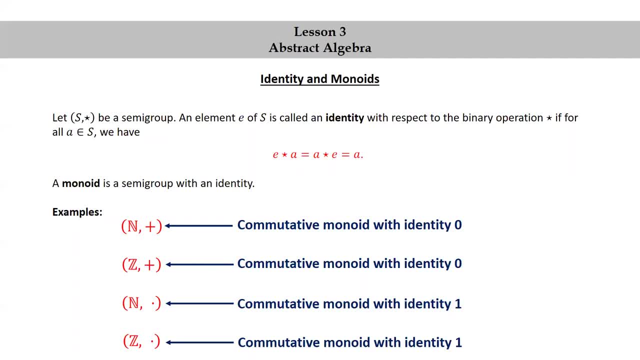 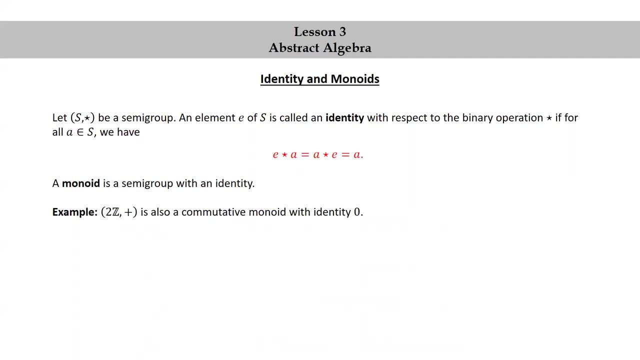 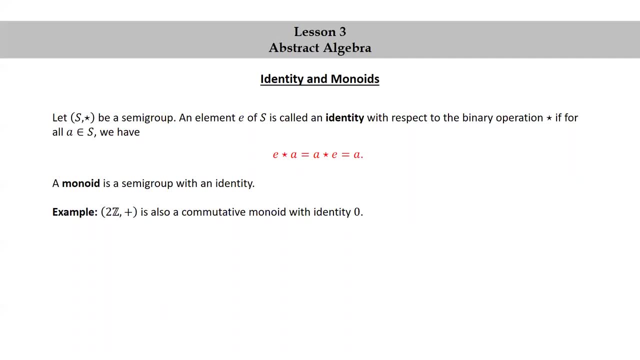 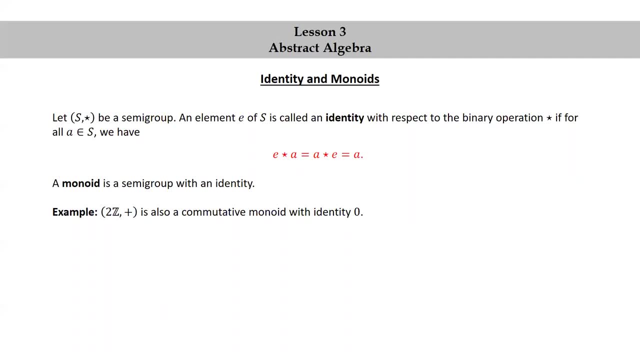 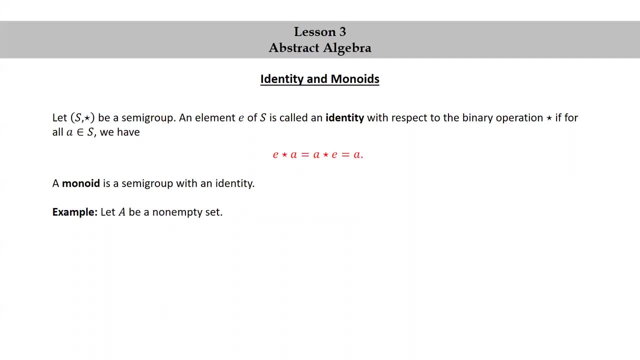 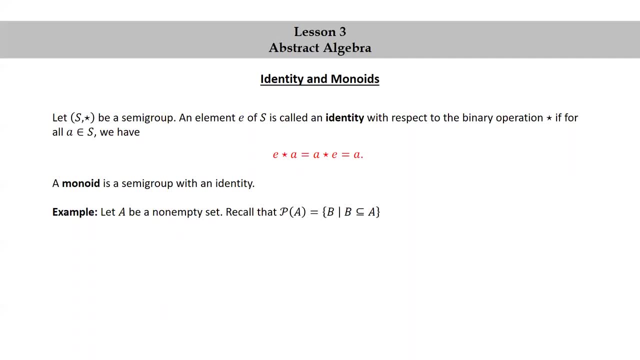 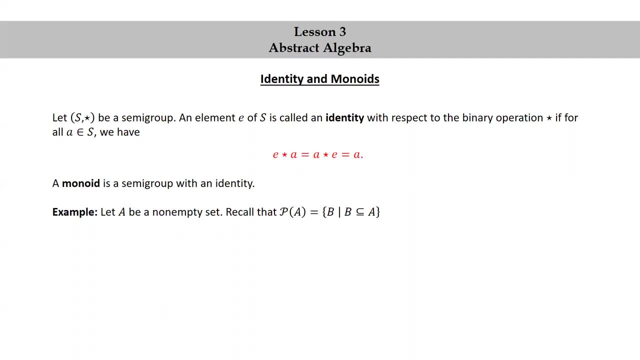 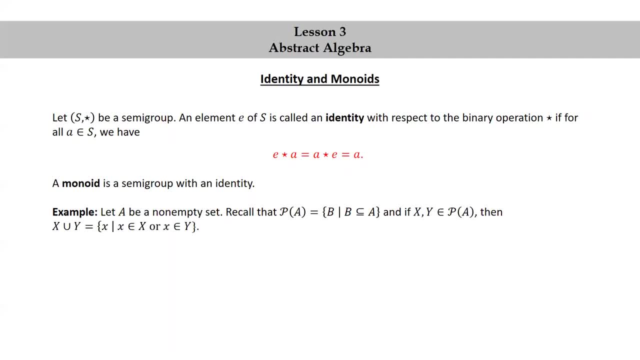 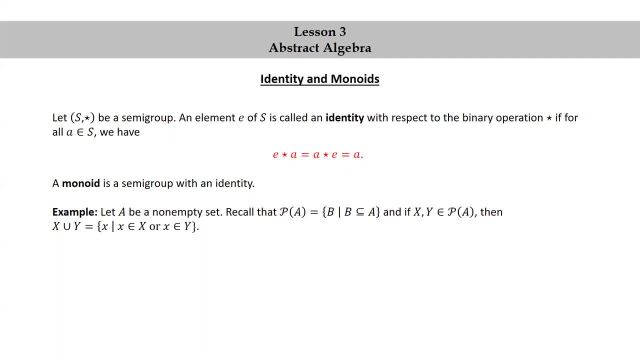 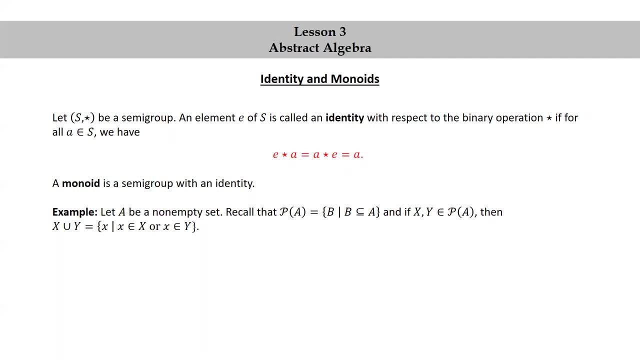 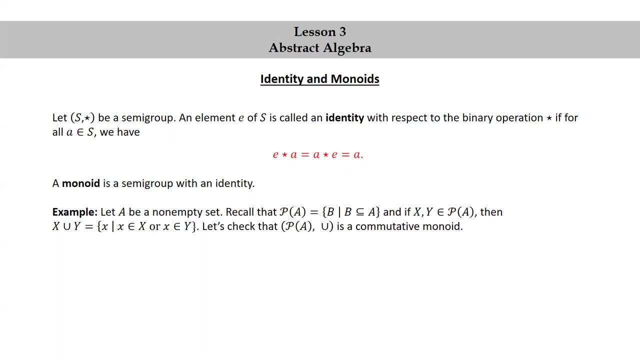 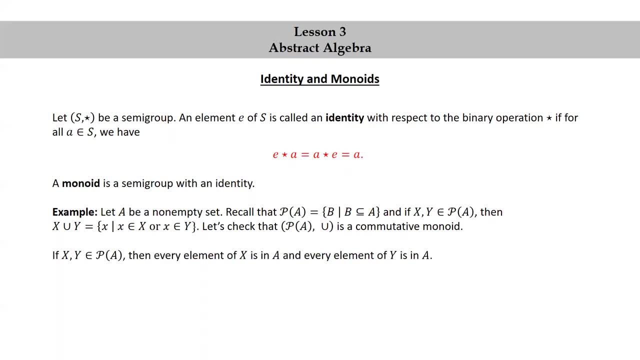 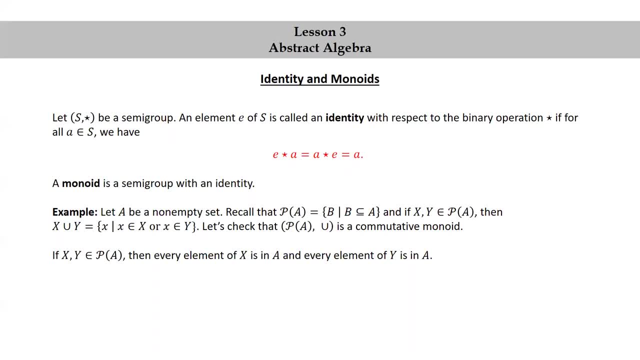 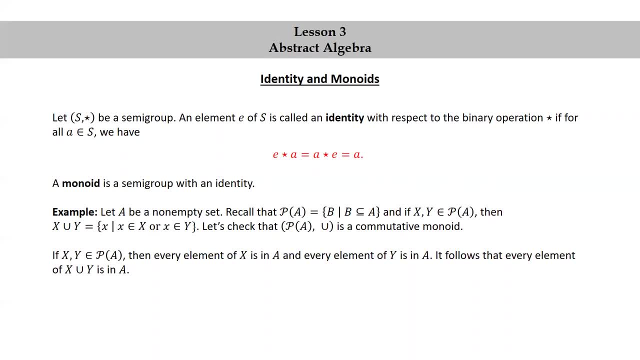 It follows that every element of X union Y is in A, so X union Y is in the power set of A. 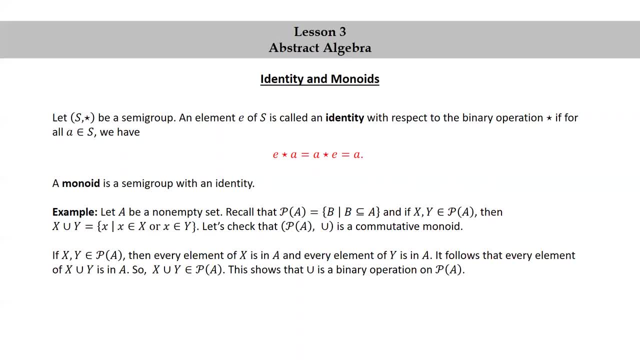 This shows that union is a binary operation on the power set of A. 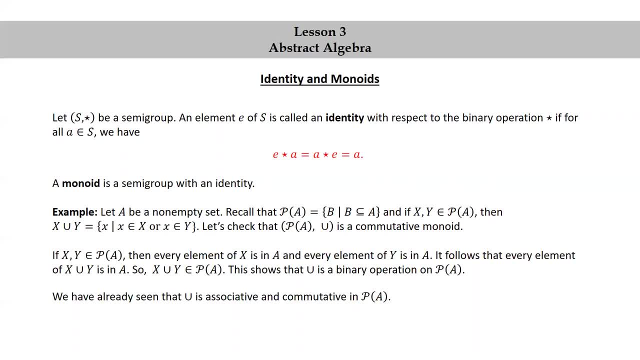 We have already seen that union is associative and commutative in power set of A. 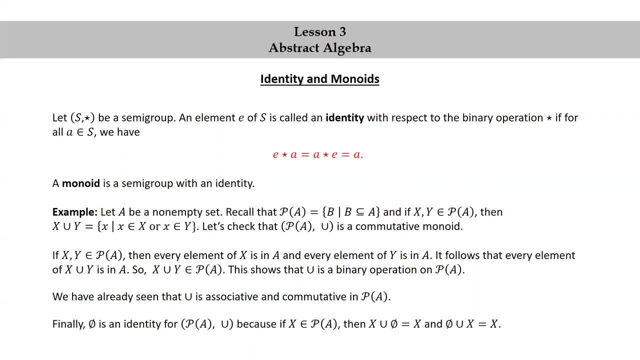 Finally, the empty set is an identity for the power set of A together with the operation of union, because if X is in the power set of A, then X union empty is equal to X, and empty union X is equal to X. 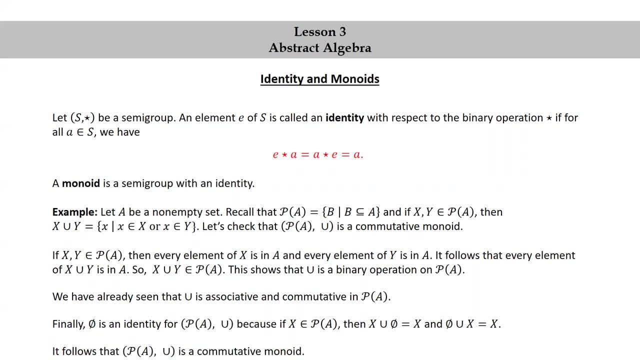 It follows that the power set of A together with the operation of union is a commutative monoid. Let's try an exercise. 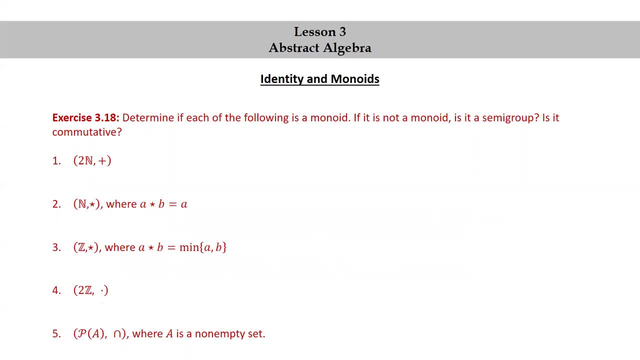 Determine if each of the following is a monoid. If it is not a monoid, is it a semigroup? Is it commutative? 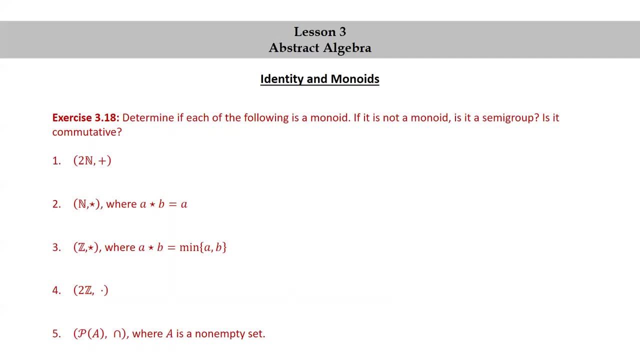 Once again, now is a good time to pause the video, try this exercise yourself, and then resume the video to check your answers against mine. 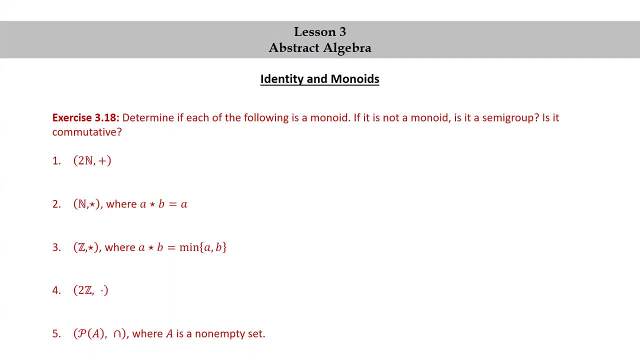 The first one, 2N, the set of even natural numbers together with the operation of addition. This is a commutative monoid with identity 0. 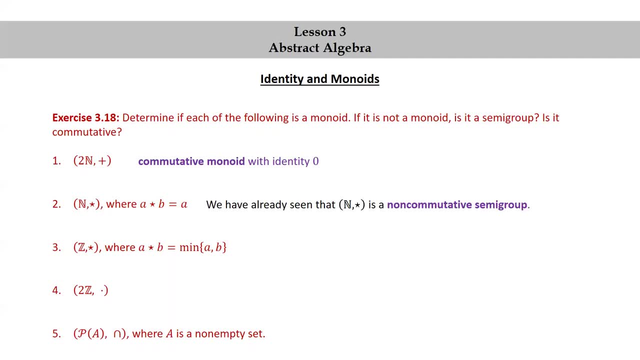 The second one, N star, where A star B is equal to A. We have already seen that N star is a commutative monoid with identity 0. N star is a non-commutative semigroup. N star is not a monoid. 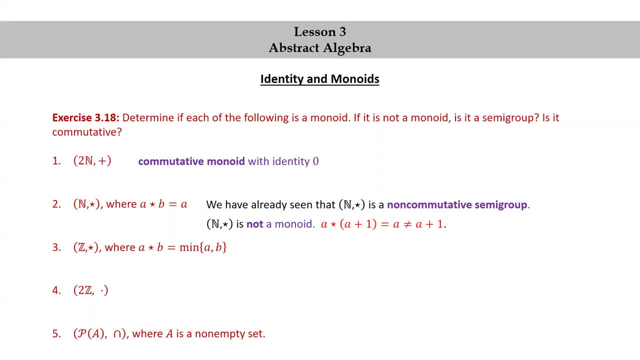 If we take any A, then we have A star A plus 1 is equal to A, which is not equal to A plus 1. So A is not an identity. 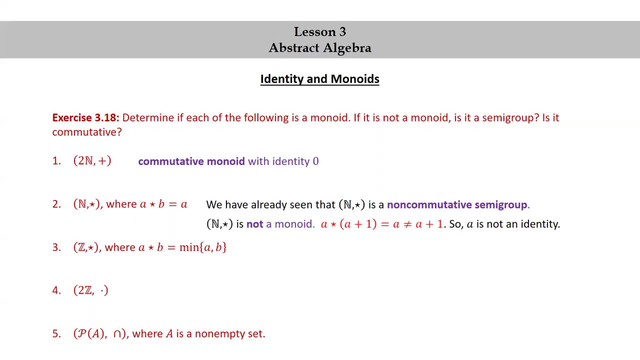 You may want to pause the video again here and look this over carefully. Many students find this argument a bit confusing until they look over. 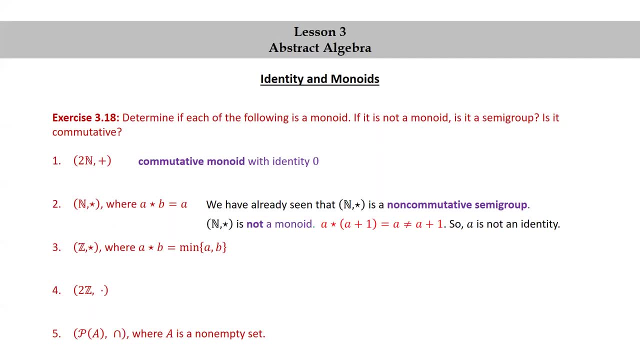 For the third one, Z star, where A star B is min A B, we have already seen that Z star is a commutative semigroup. Z star is not a monoid by the same reasoning as in number 2. 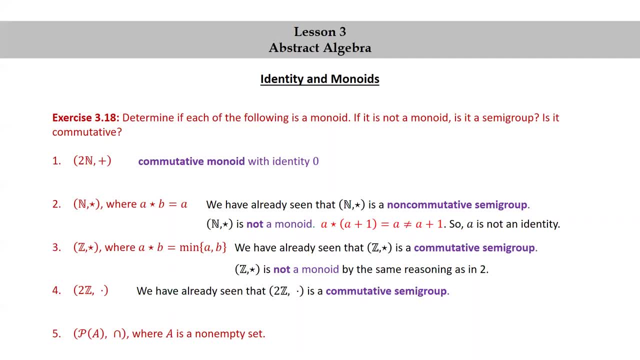 2 Z times is a commutative semigroup. We've already seen that. 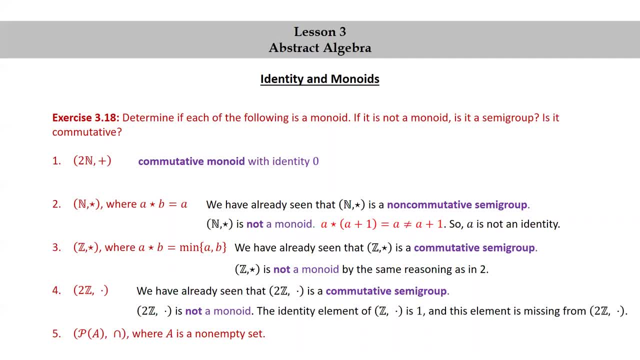 But it's not a monoid. The identity element of Z together with multiplication is 1, 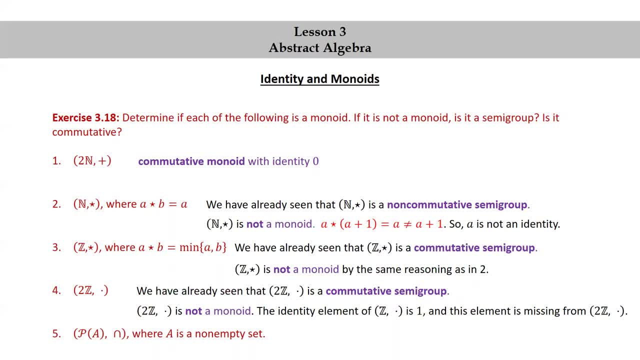 and this element is missing from the set of even integers together with multiplication. 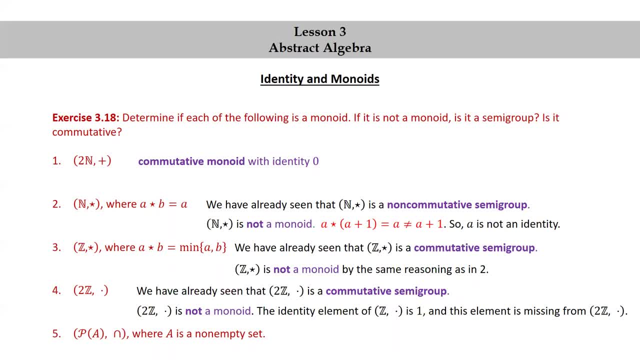 The power set of A together with the operation of intersection, where A is a non-empty set, this is a commutative monoid with identity A. Let's check the properties carefully. Closure. 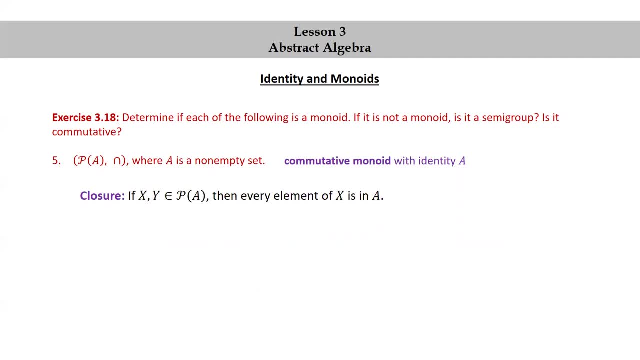 If X and Y are interlinked, then every element of X is in A. Since every element of the intersection of X and Y is an element of X, it follows that every element of the intersection of X and Y is in A. So the intersection of X and Y is in the power set of A. 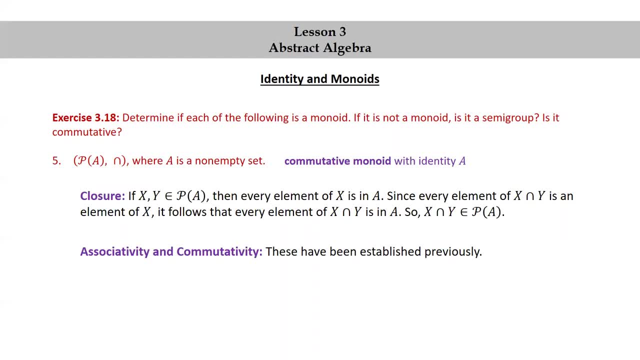 Associativity and commutativity. These have been established previously. Identity. 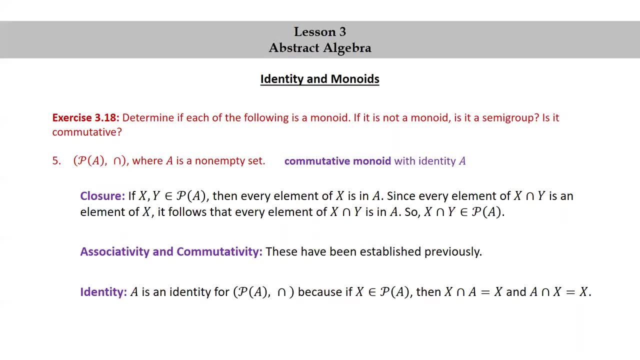 A is an identity for the power set of A together with the object. 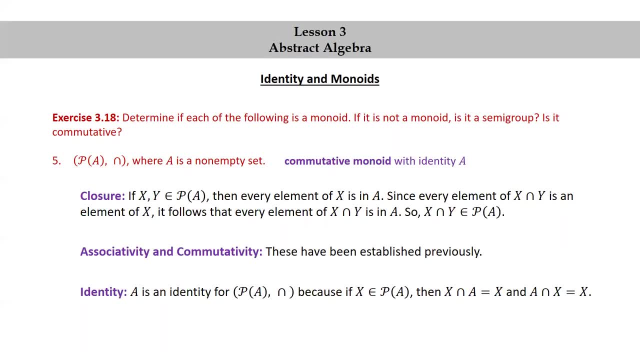 It is an operation of intersection. Because if X is in the power set of A, then X intersect A is equal to X, and A intersect X is equal to X. 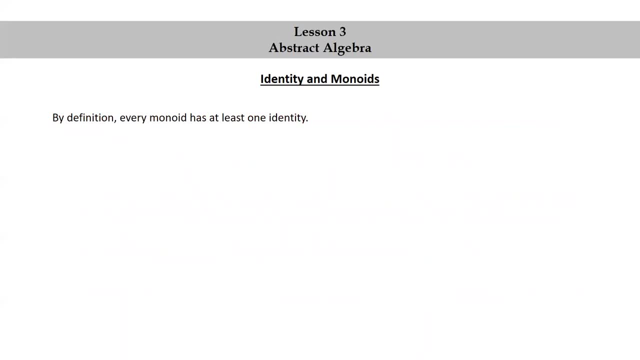 By definition, every monoid has at least one identity. It is natural to ask if a monoid can have more than one identity. We will now discuss why this cannot happen. Monoid fact one. In any monoid, M star, the identity is unique. Analysis. 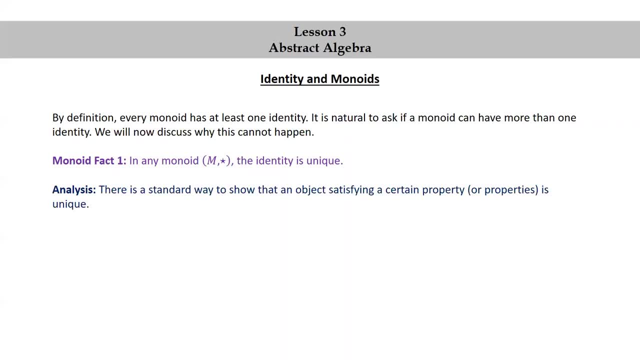 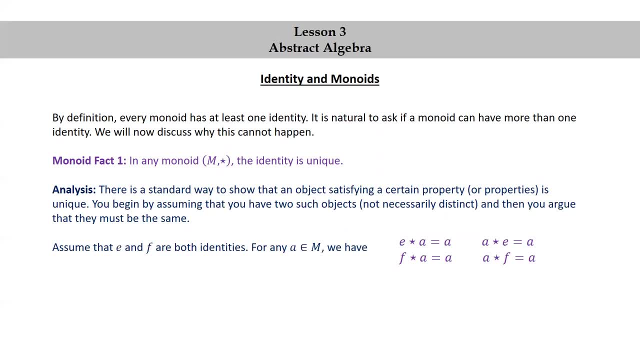 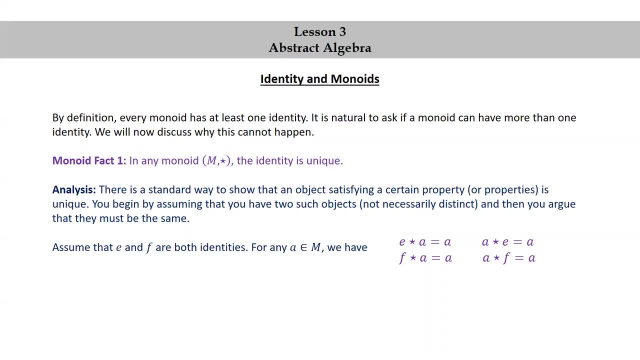